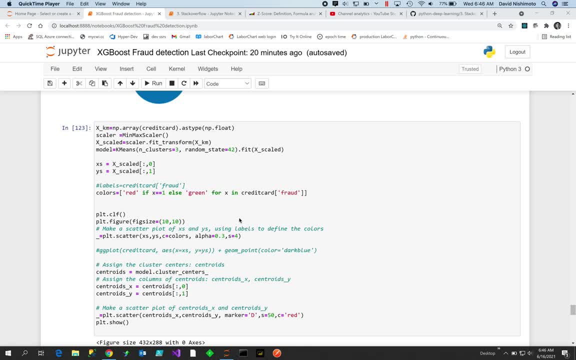 well on my machine for some reason, so i won't be demonstrating that, but i will be showing you kdmean. okay, so what we do is we we're going to take the credit card data frame and we're going to convert that into a numpy array and as a float, then we'll take our min max scalar and we'll transform that. 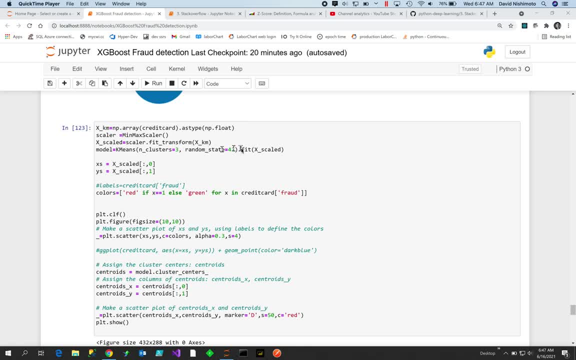 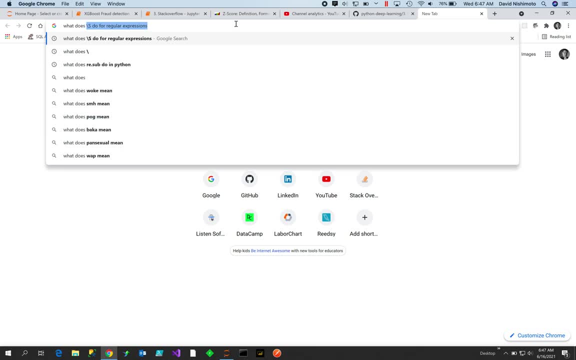 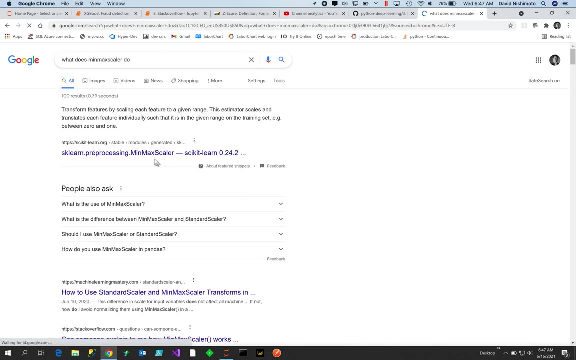 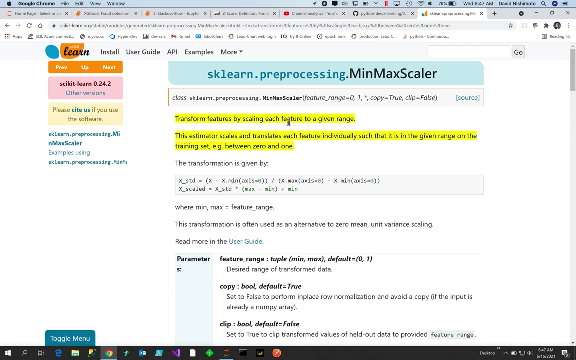 and that will then create us an x scaled. let's see. let's go over here real quick. what does min max scalar do? okay, so that'll, that'll give you an idea. says transforms features by scaling each feature to a given range. this estimator scales and translates. 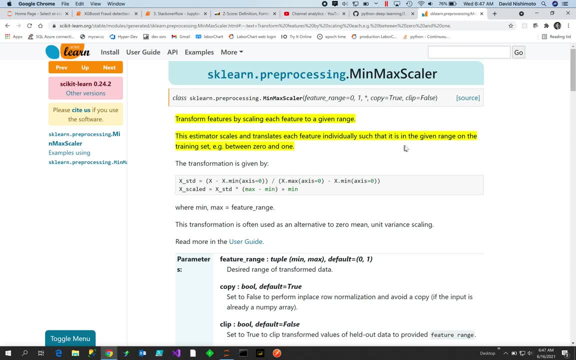 each feature individually such that it is in the given range on the training, set between zero and one. and then this is the formula that's transformed, so it gets the. it takes the x minus the x and the x min divided by x max, divided minus x min, and then you have the standard deviation times the min. 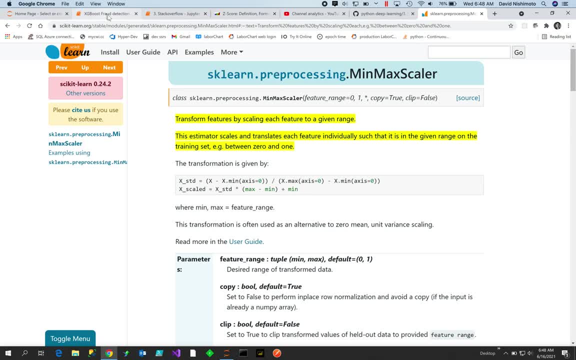 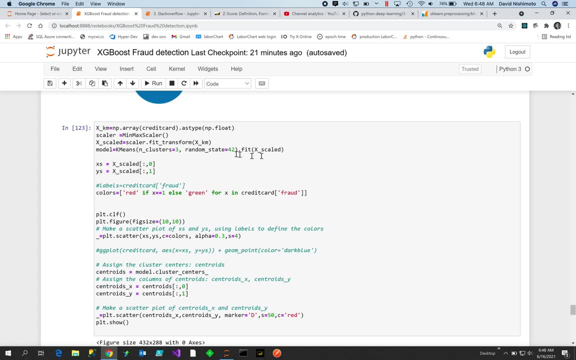 minus the max, plus the min. so that's what the that function is doing. you could create your own if you wanted, okay? so now that we have the uh x scale, we'll, we'll, we'll set that as we'll fit it, and then we'll transform it and then that'll create our x scale, and then we feed the x scale into our k. 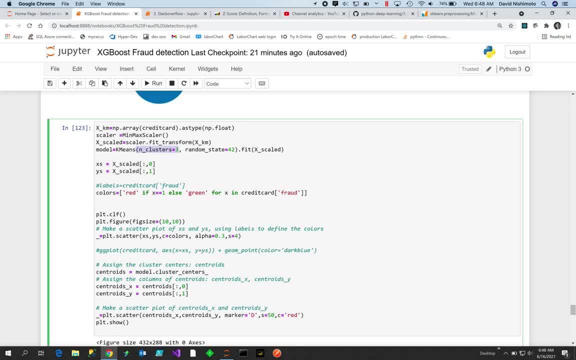 so that's what that means. you have to know the number of clusters here, and i'm going to show you the elbow technique that is used to determine that cluster count. okay, once we have that, then we're going to get x scaled. we'll have an x and a y component, so the first, the first value, will be: 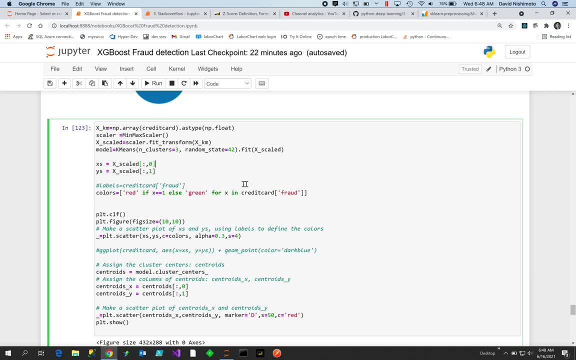 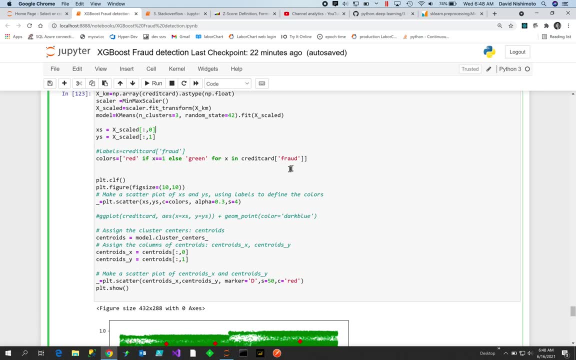 for y will be zero and the second one will be one for y. okay, i just set some random colors here. so if x is one red, otherwise it'll be green and i'll show you that in a moment. but it's just going to go through the credit card fraud and and set up my colors for my scatter plot. so then, when my scatter plot i 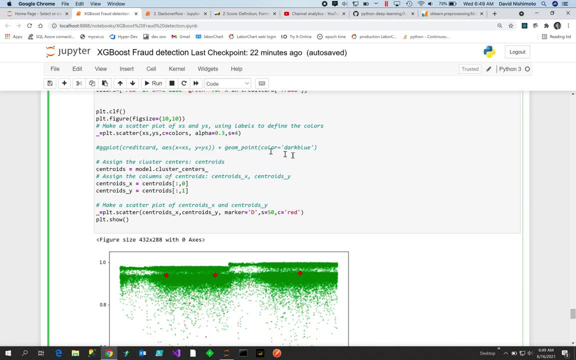 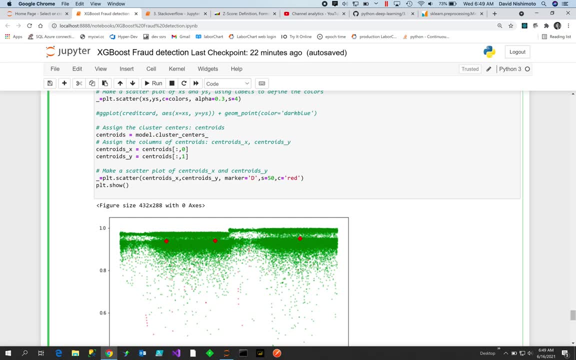 pass in my x and y and my colors. now what we need to do is we need to grab from the k means our cluster center. we can get our cluster centers, uh, and we can also get our um. we can get the coordinates on those cluster centers and i'll show you that in a minute. 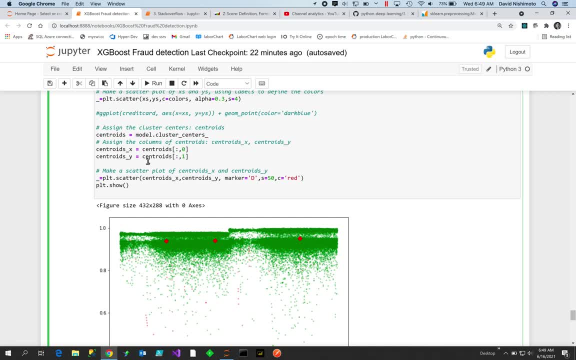 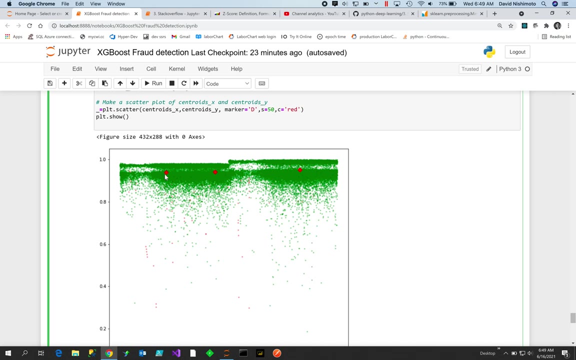 so once we have the centroids, uh, we can then uh, get their x and y, and then in another scatter plot we can, we can plot out the x and y, and we'll just use this marker d and the color red. so what you can see here then is we have three centroids and then we have these little red dots here represent. 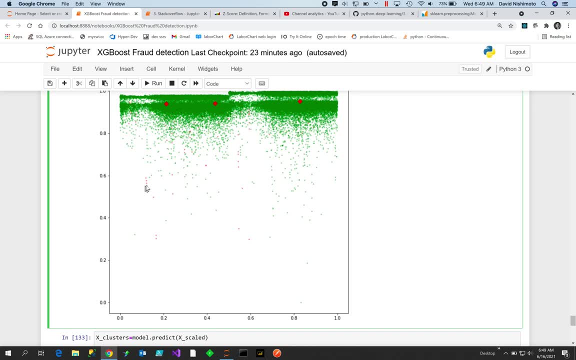 the fraud cases and you can notice that in the plotting of it that there is a little bit of a gap between the two of them. so you can see that there's some groupings like you can see, like there's some grouping here, there's some grouping here, there's some grouping here, and those are uh. 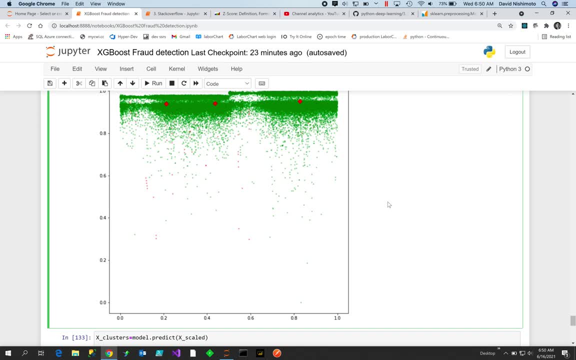 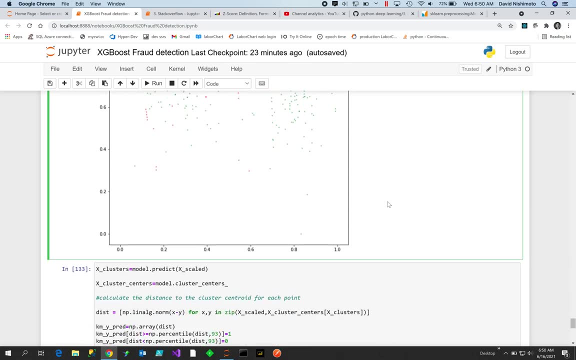 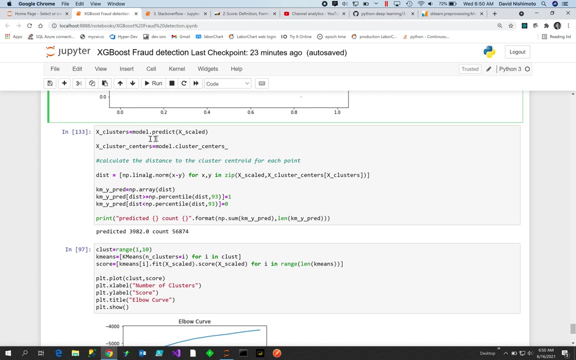 groupings that you know you could send over to the fraud department and extract that information. that's what the db scan does, is it provides you a distance equation and i'll show you that in just a moment. okay, so here is what you do. you get you. you would get our clusters on the model. k means predict. 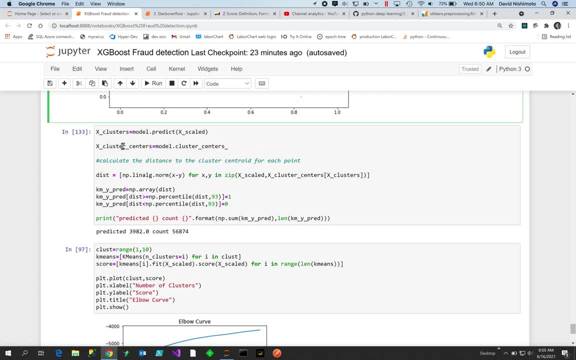 ном, they get the zodiacal coordinates being the set of all of the clusters, and then the data that they bring up will give us the clusters, and then we can also get the cluster centers. so we have the clusters and cluster centers, so combined with clusters and cluster. 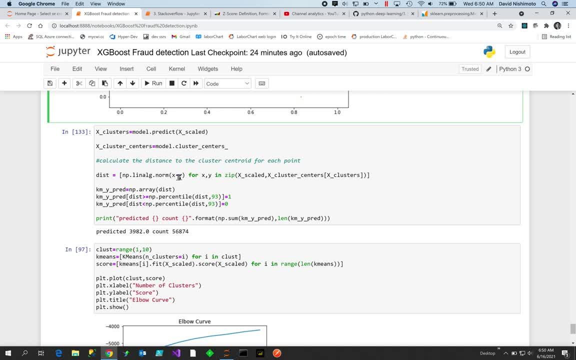 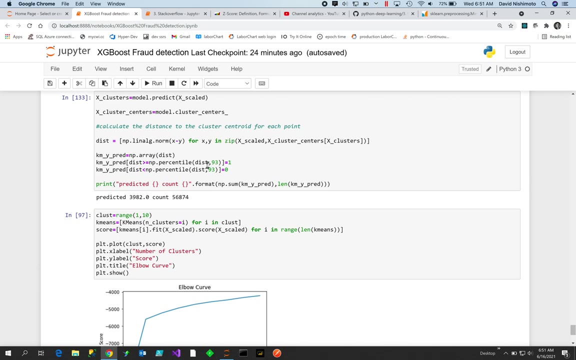 centers. we're going to zip that with the x scale and then we can. we can get a tuple of x and y and then we can do a normalization- x minus y- and that will create a distance equation. Okay, so then what we do here is we're looking for outliers. 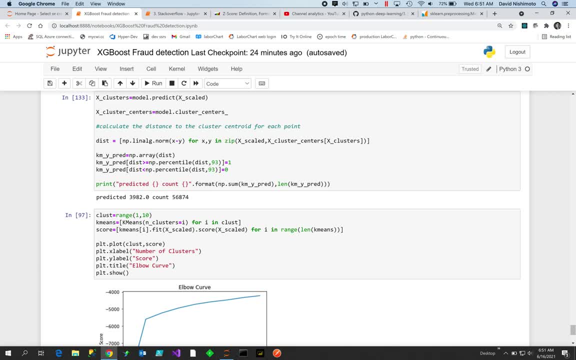 and so we will do the percentile where the distance is greater than the 93rd percentile, and then we'll mark that as a 1.. Otherwise it will be marked as 0, and then we can do our prediction. So our prediction here would be that there were 3,982 fraud cases out of 56,874.. 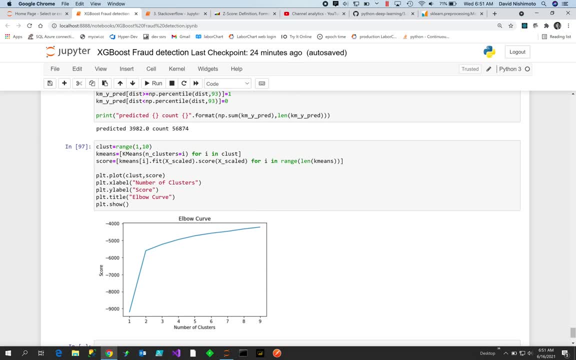 Okay, the way I got the number of centroids I was going to follow is I have a k-means cluster here and I get the k-means and I'm going to look at different clusters where it's going to vary from 1 to 10.. 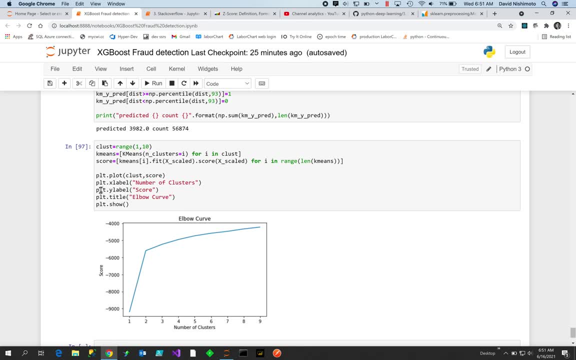 So you can see, here I've got 1 to 10.. And what I'm looking for when I fit with the k-means is: I'm going to fit it, I'm going to then score it and I'm looking to plot the score. 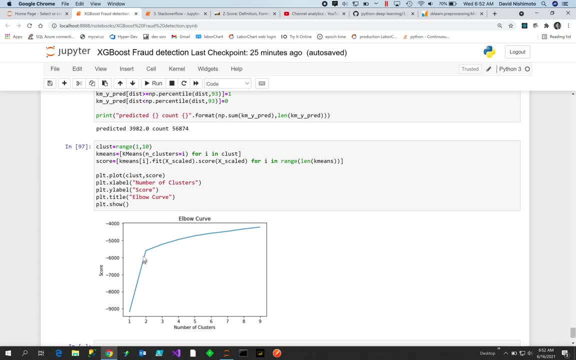 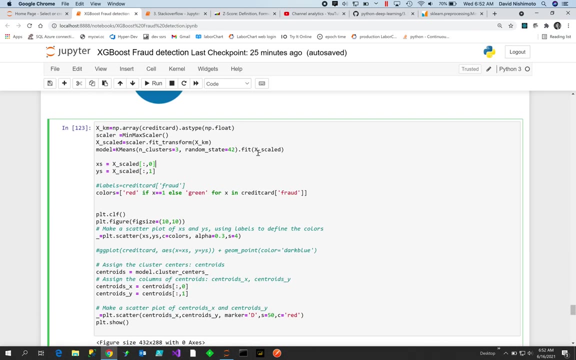 So you can see at 1, centroid 2, centroid 3.. So it's possible that this elbow turned right here on 2 or 3.. And if we come back to the data here and we ran this, See, I'm not sure I can do that at this point. 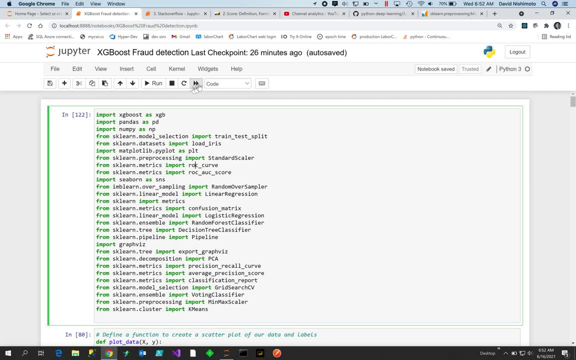 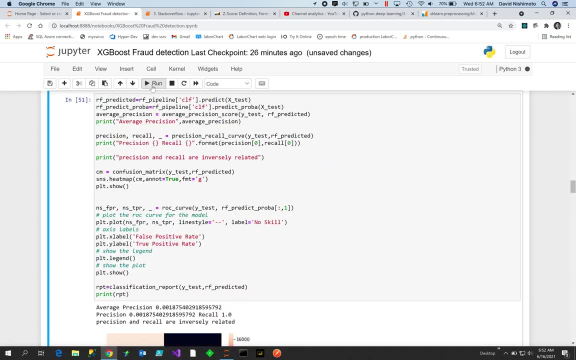 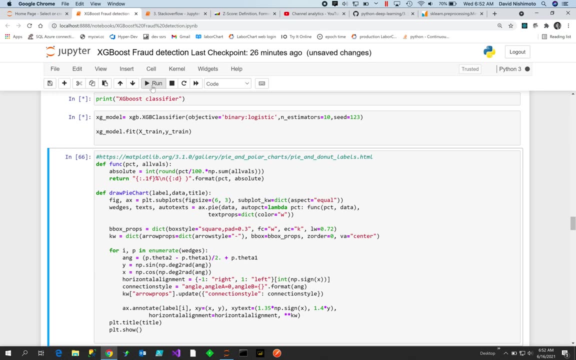 No, because I have to run them all. Okay, Let's just kick it off, It doesn't take that long. This is all the code that we've covered in previous YouTubes, So you can find the one on XGBoost fraud. 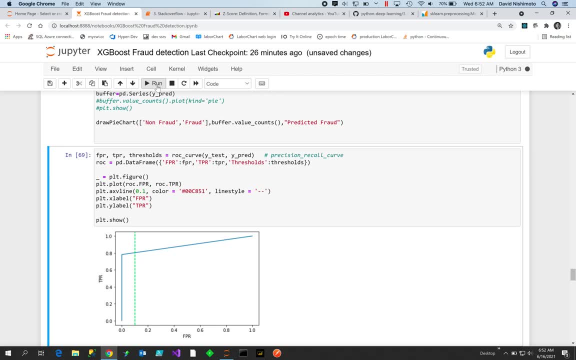 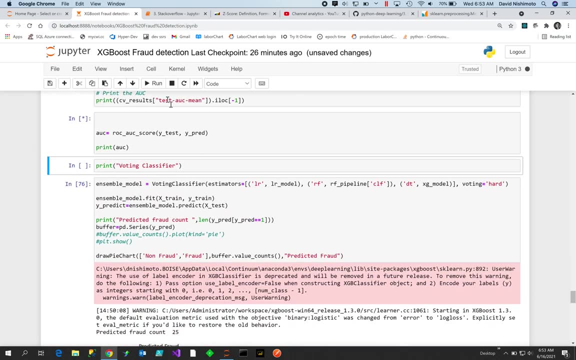 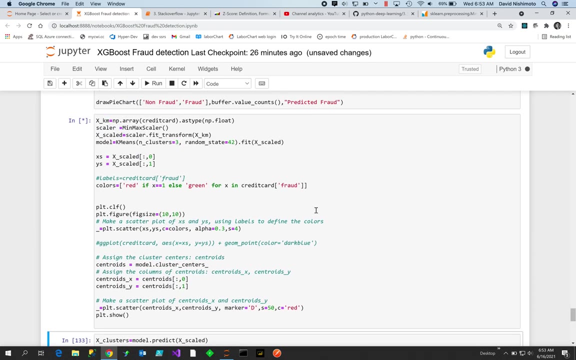 and we'll see what happens. You can go over that video if you're interested in how that works. Okay, Click pass here. Get past my validation. The validation is going to take a little while Loading classifier. Okay, So at some point that's going to run. 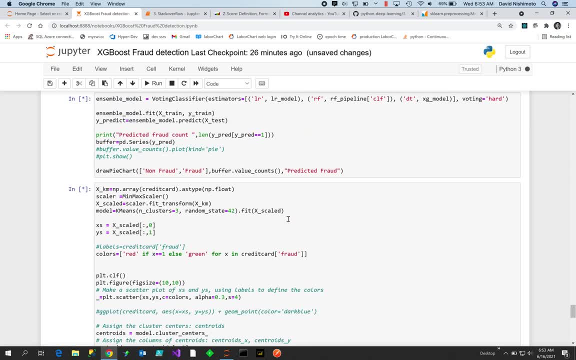 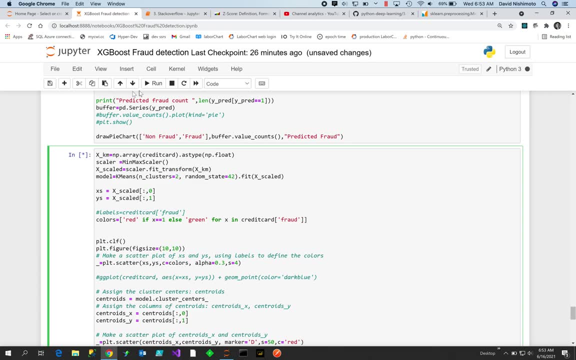 So yeah, So we can change the centroid- Let's see Where was it Here. We can change that to 2 and then run that again. So that's what I would have done, And then you can see that there would be two clusters and how that would group. 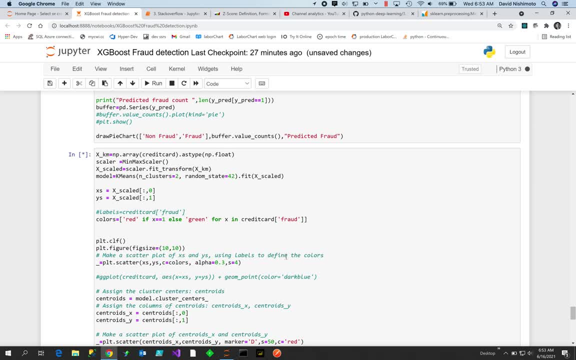 But when I did that, it looked better with three clusters. It looked like the data was grouping better with three clusters. Okay, Well, download my code and run it and try it out.